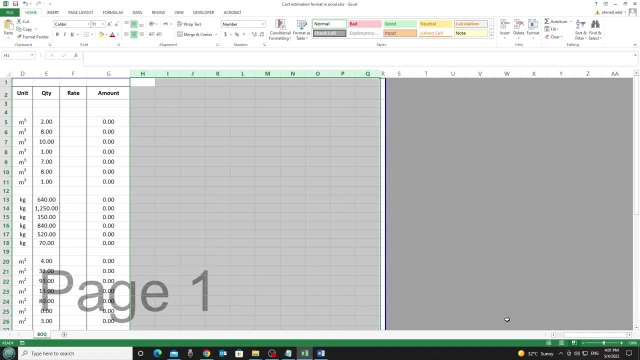 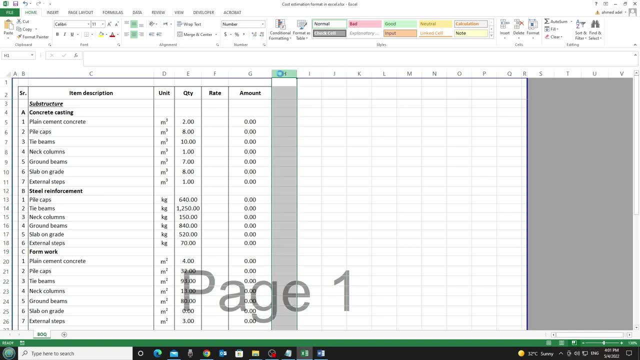 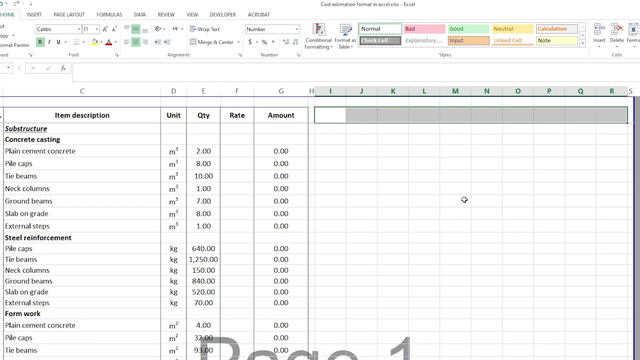 10 columns here, and I'll tell you why in a moment. So let's just adjust them like that And let's have this, Let's have one more column just to separate our schedule from the BOQ itself. So here I want to make the rate breakdown analysis And what I want to do. 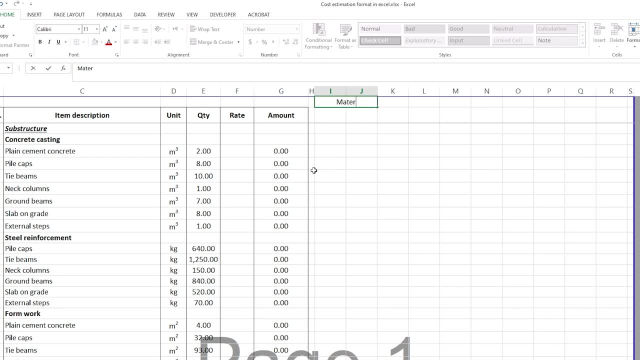 I want to start with materials. So here I'll put materials and here I'll put equipment, And here I can put the manpower, And these are the cost elements that we have, And here I can put subcontractor. So for each of these four cost elements I have two columns, And then the last one will be. 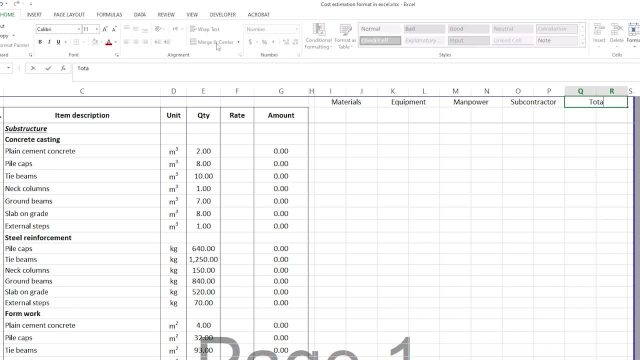 the total, And I'll explain what is that in a moment. So this is the first thing. Second thing I want to write here: rate, then amount. So for each of these cost elements I have rate and amount, even for the total as well. So this is what I have done so far. I'll remove. 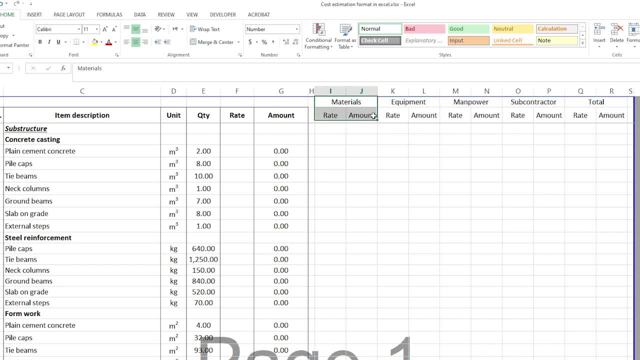 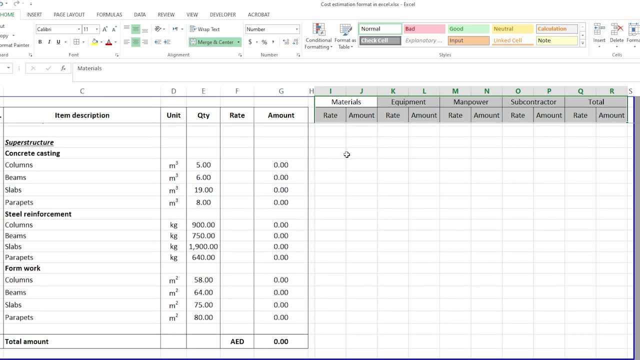 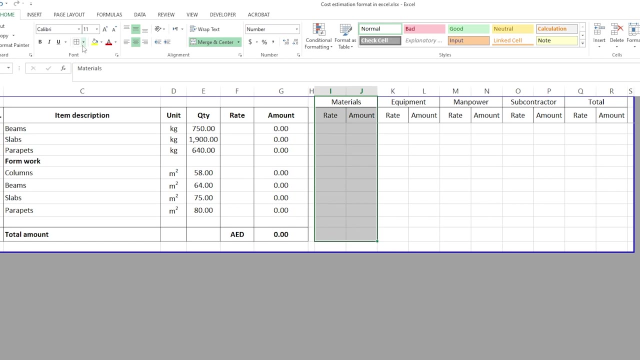 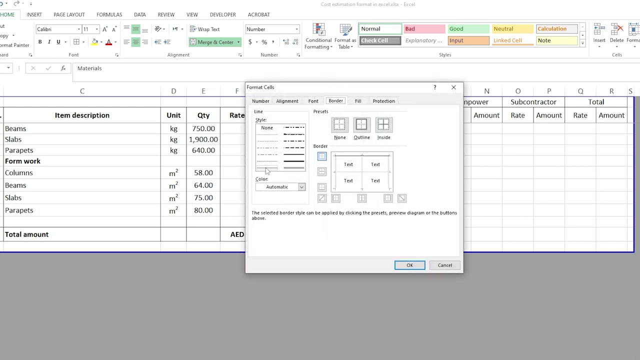 this bolt Like that, Then let's have these cost elements with all borders And now let's go down like that, Okay And okay, starting from the materials here up to this sill. I can just go here and go to more borders And what I want I want from left and right. I want solid lines, So I'll just select. 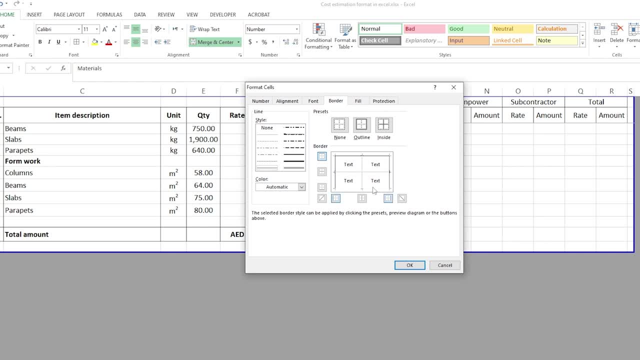 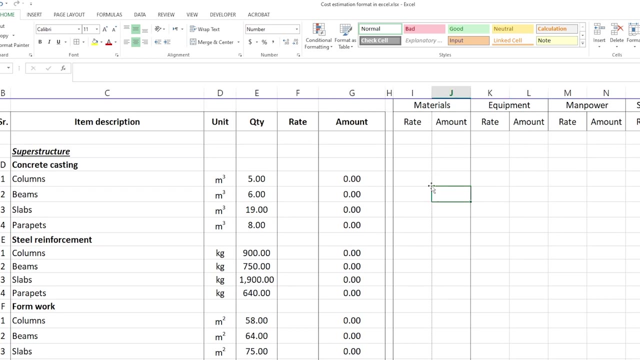 the solid line here And I'll make this a solid line, And this is a solid line, And below also a solid line, And I need a dotted line here in the middle And I'll click OK. Nothing happened. I don't know why, or actually it came here. there is a dotted line. 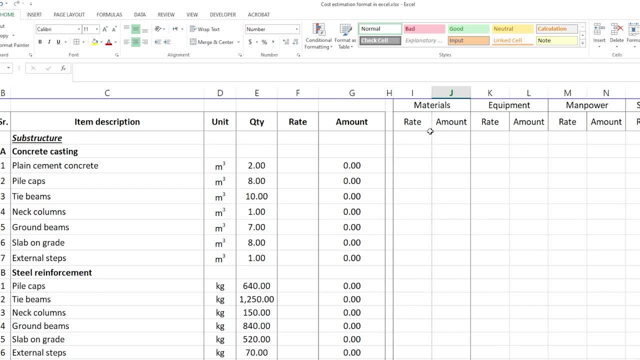 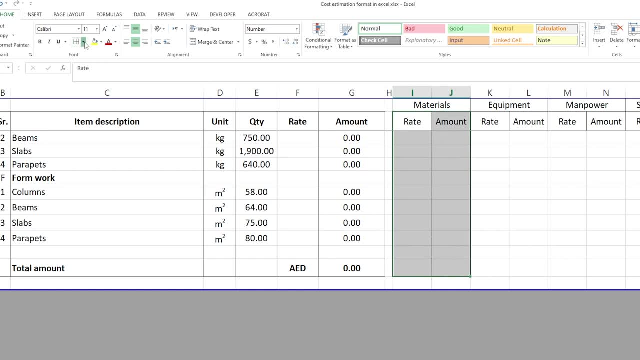 And here there is a solid line. and here there is a solid line. So let's just confirm this dotted line in the middle. So again, I selected the full range and I'll go here to more borders And I'll make sure that I have a dotted line in the middle. 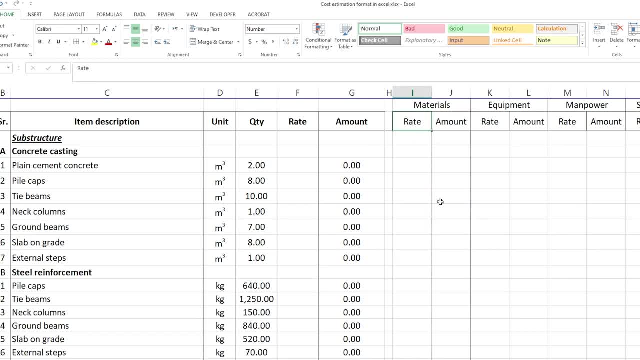 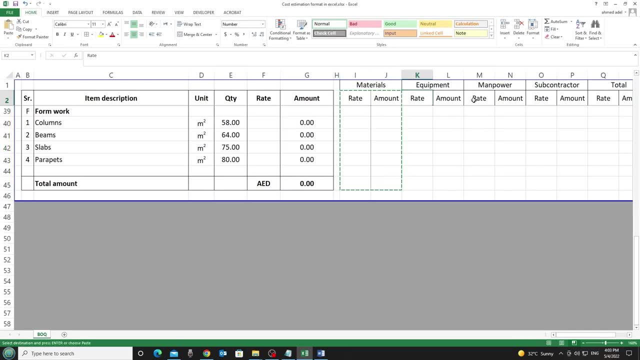 Okay, so there is a dotted line in the middle now, And all I have to do is to just copy this range from this cell up to down. I'll copy that and I'll paste it here and here and here and here as well. 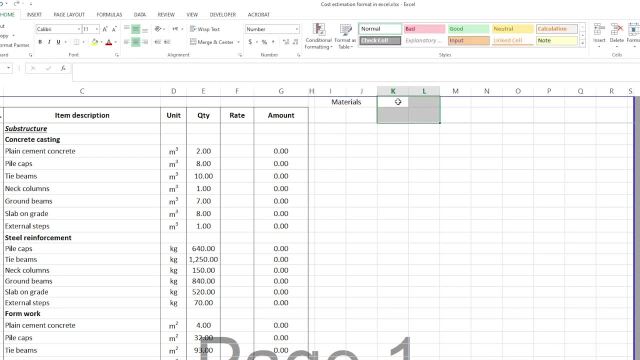 materials, and here I'll put equipment, and here I can put manpower, and these are the cost elements that we have, and here I can put subcontract. so for each of these four cost elements i have two columns, and then the last one will be the total, and i'll explain what is that in a moment. so this is the first thing. second thing i want to write: 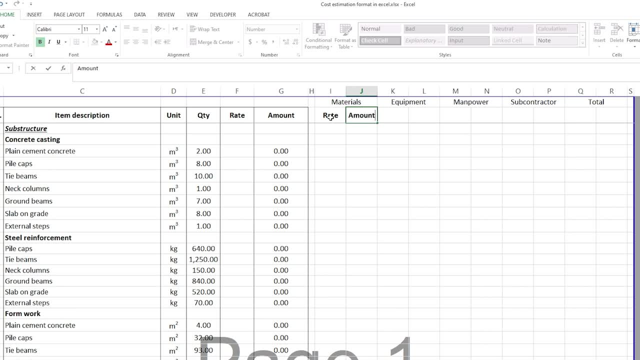 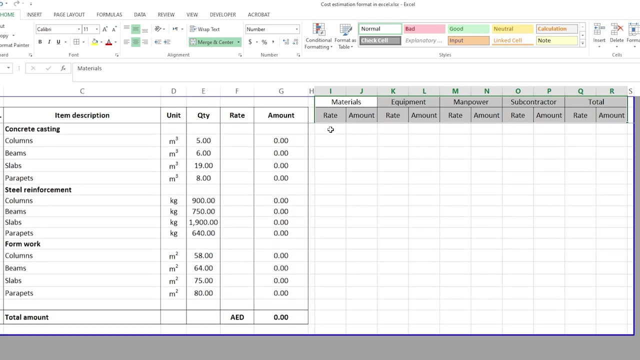 here: rate, then amount. so for each of these cost elements i have rate and amount, even for the total as well. so this is what i have done so far: i'll remove this bolt like that. then let's have these cost elements with all borders and now let's go down, like that. okay and okay. starting from the 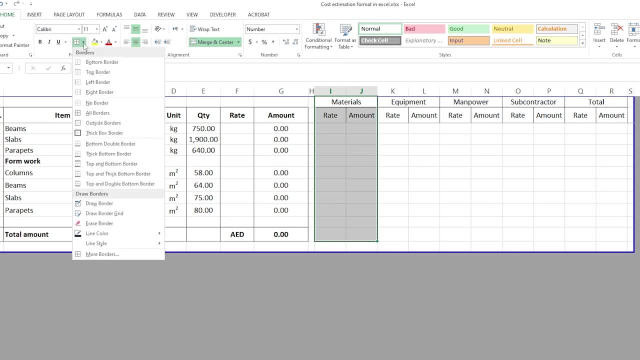 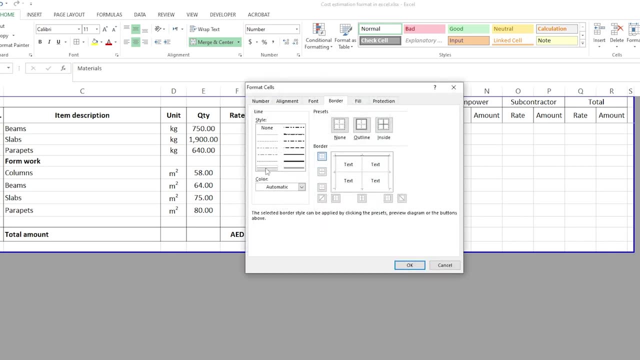 materials here up to this sill. i can just go here and go to more borders and what i want- i want from left and right, i want solid lines. so i'll just select the solid lines and then i'll go to the line here and I'll make this a solid line and this is a solid line and below. 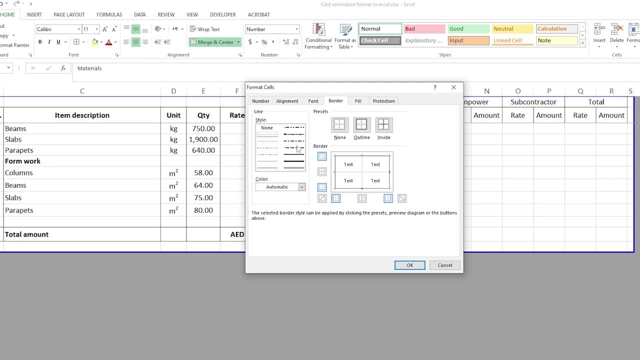 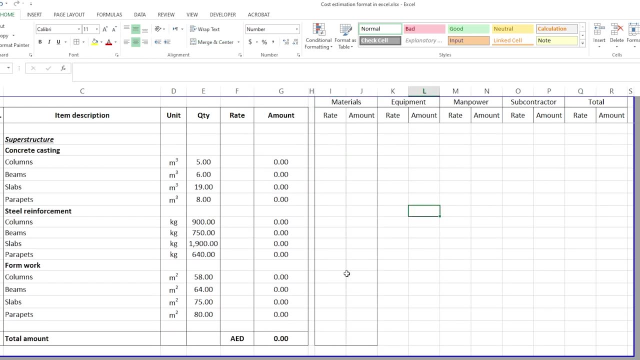 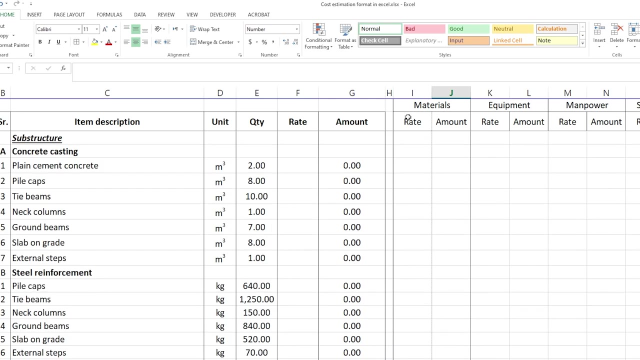 also solid line, and I need a dotted line here in the middle and I'll click. OK, nothing happened, I don't know why, or actually it came. here there is a dotted line, and here there is a solid line, and here there is a solid line. so let's just. 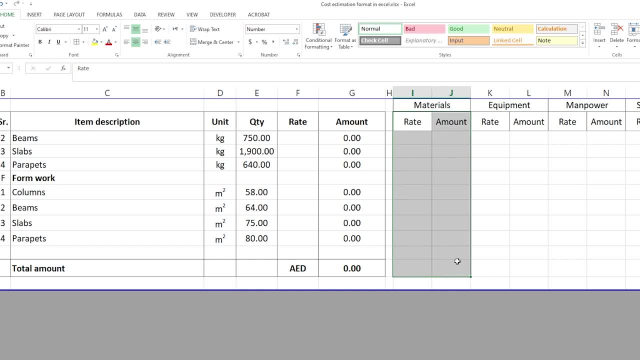 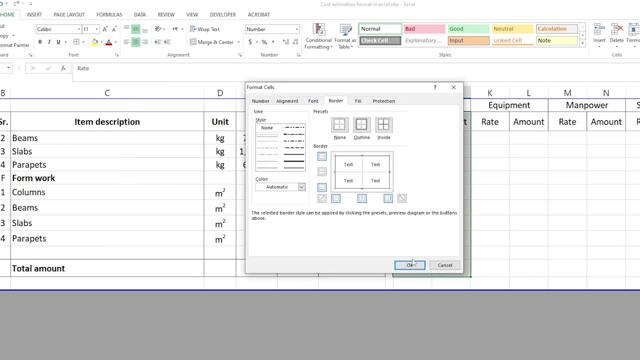 confirm this dotted line in the middle. so again, I selected the full range and I'll go here to more borders and I'll make sure that I have a dotted line in the middle. okay, so there is a dotted line in the middle now and all I have to. 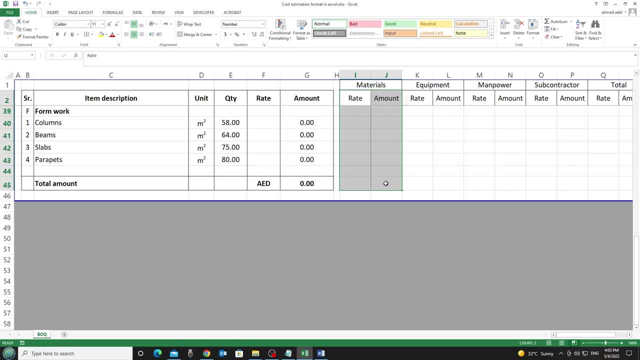 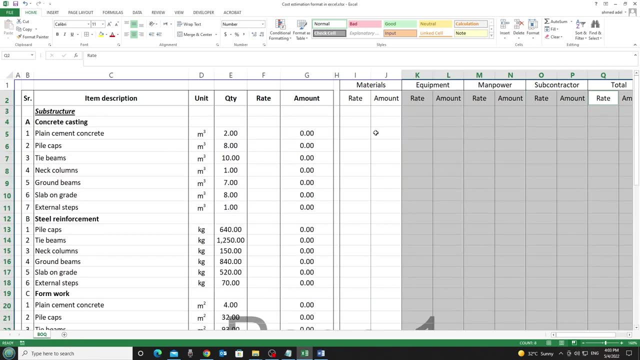 do is to just copy this range from the, from this cell up to down. I'll copy that and I'll paste it here and here and here and here as well. so what I have now? I have something that looks like this, so I'll just zoom out a little bit. so this: 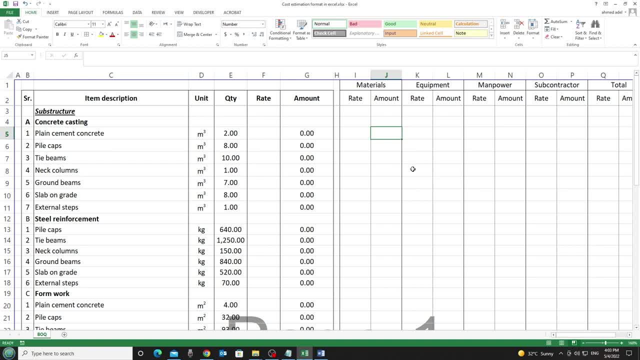 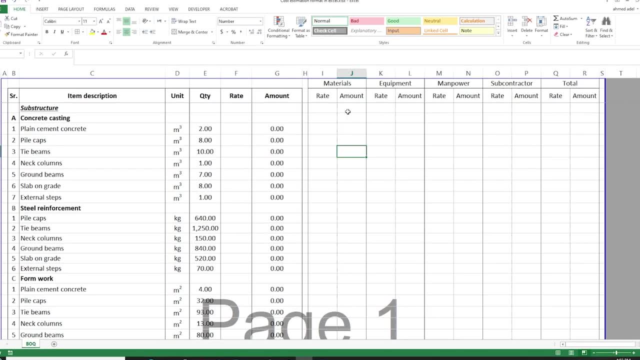 So what I have now? I have something that looks like this, So I'll just zoom out a little bit. So this is what we have. We have the materials, equipment, manpower, subcontractor and total, And we have rate and amount for each of them. 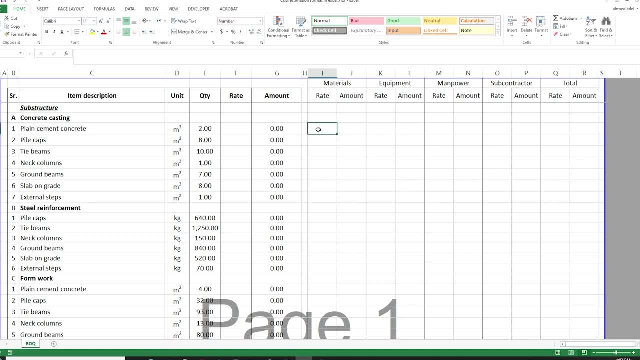 So I'll start with the material. Whatever rate I'll put here, this rate will be for the material And whatever amount will come here will be the rate of the material multiplied by the quantity of the material. So I'll say the amount is equal to the quantity. 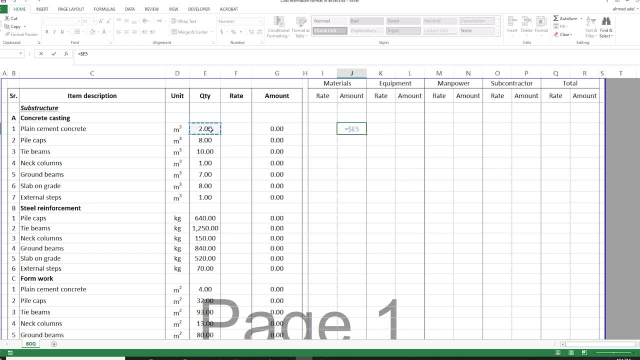 But don't forget the dollar sign for the column. So dollar E5 multiplied by this rate, which is the material rate here. OK, so if I copy this formula and paste it here, what happens? I am multiplying the rate of the equipment by the quantity. 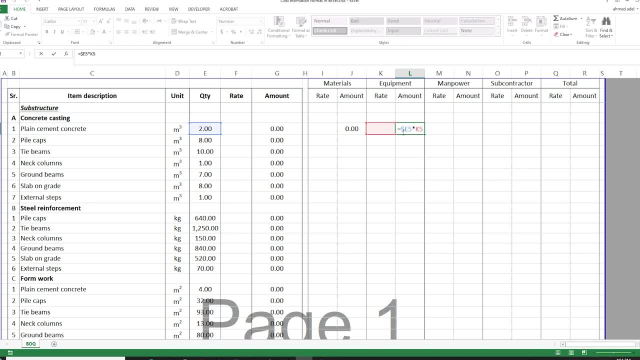 You see, the column quantity is fixed because of the dollar sign next to the E column. OK, so again, I'll copy this and I'll put it here and here and here, Then I'll press enter. So what happens now? I am multiplying the rate of the manpower by the quantity and multiplying the rate of the subcontractor by the quantity. 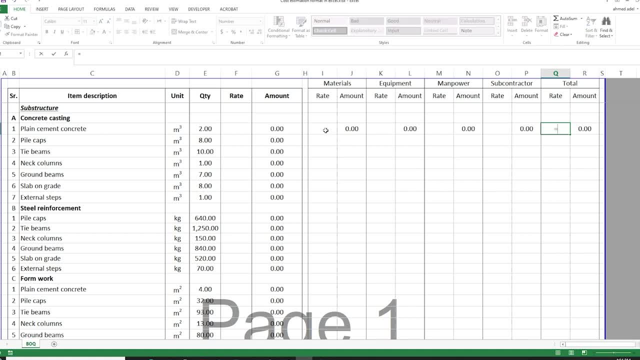 And actually the total rate will be equal to the material rate plus equipment rate, plus manpower rate, Plus subcontractor rate and enter And the total amount is equal to the total rate multiplied by quantity. So I have this line now, OK, and I'll copy this line and I'll paste it everywhere else. 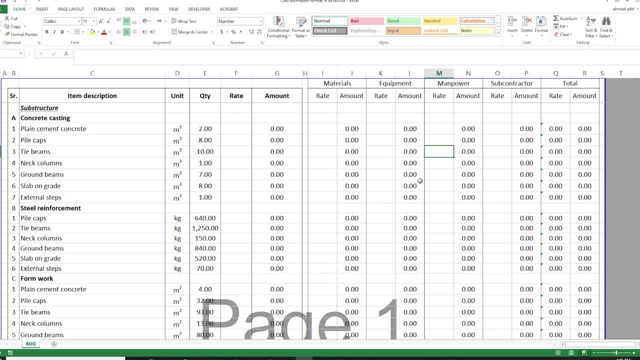 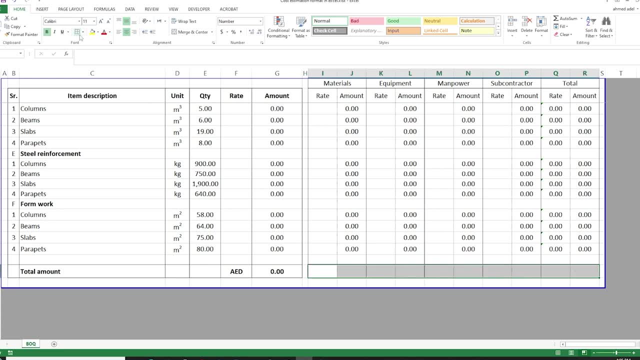 Done. So now I have this format. All what you need now is to start estimating the cost, And To do this, let's have some total here. So again, more borders, and I'll put a solid line on top. So I have a solid line here on top and click OK. 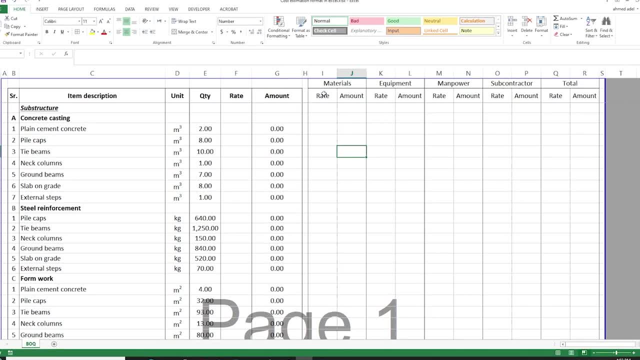 is what we have. we have the materials, equipment, manpower, subcontractor and total, and we have rate and amount for each of them. so I'll start with the material. whatever rate I'll put here, this rate will be for the material and whatever amount will come here will be the rate of the material multiplied by 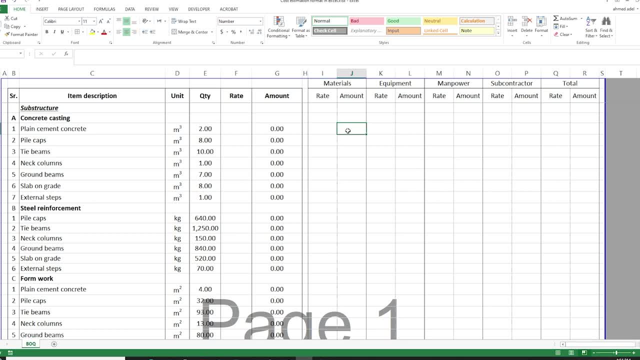 the quantity of the material. so I'll say the amount is equal to the quantity, but don't forget the dollar sign for the column. so $ cinco x this rate, which is the material rate here. okay, so, because those are my values. so if i copy this formula and paste it here, what happens? i am multiplying the rate of the equipment. 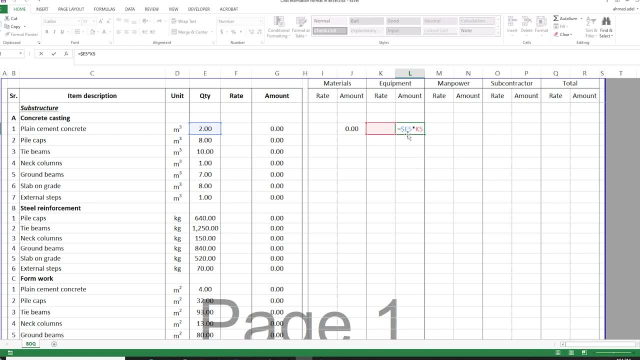 by the quantity. you see, the column quantity is fixed because of the dollar sign next to the e column. okay, so again, i'll copy this and i'll put it here and here and here, then i'll press enter. so what happens now? i am multiplying the rate of the manpower by the quantity and multiplying the. 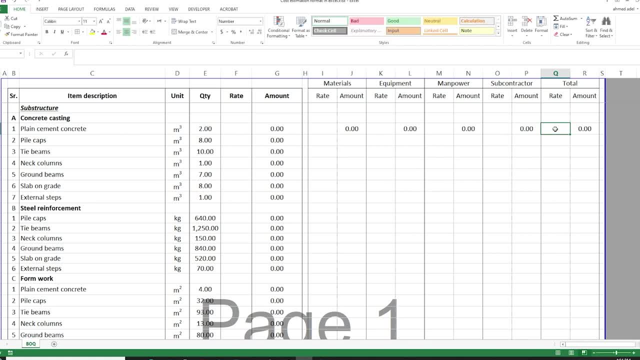 rate of the subcontractor by the quantity, and actually the total rate will be equal to the material rate plus equipment rate, plus manpower rate, plus subcontractor rate and enter and the total amount is equal to the total rate multiplied by quantity. so i have this line now. 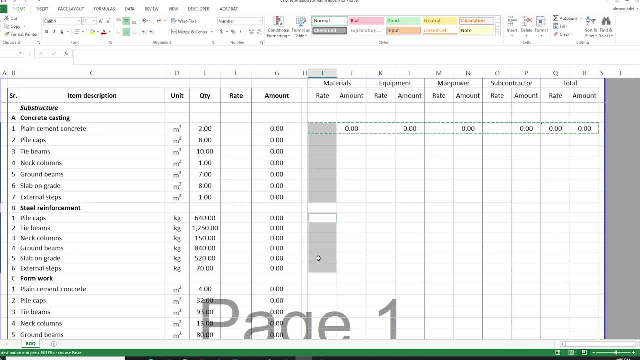 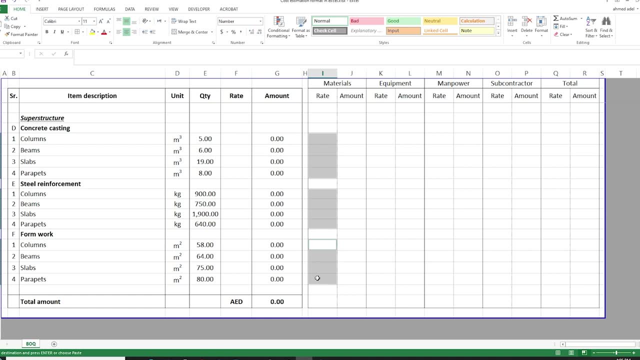 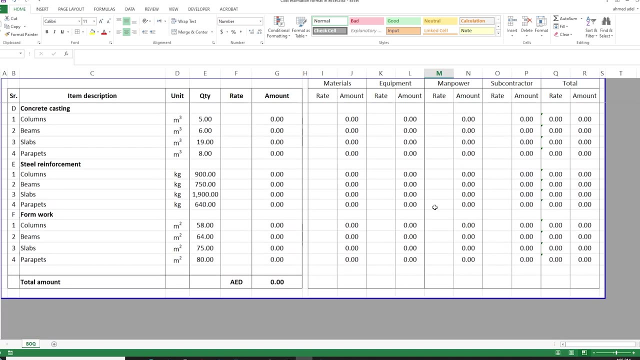 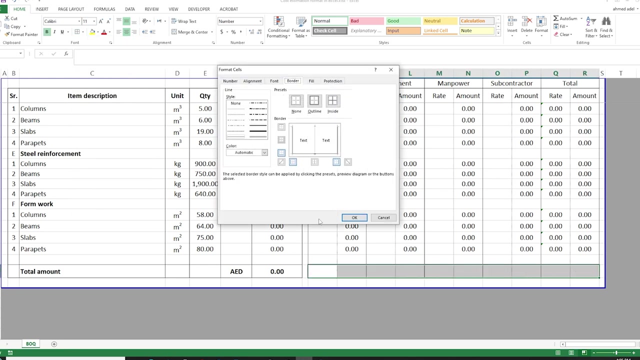 okay, and i'll copy this line and i'll paste it everywhere else. done so, now i have this format. all what you need now is to start estimating the cost and to do this, let's have some total here. so again, more borders, and i'll put a solid line on top. so i have a solid line here on top and 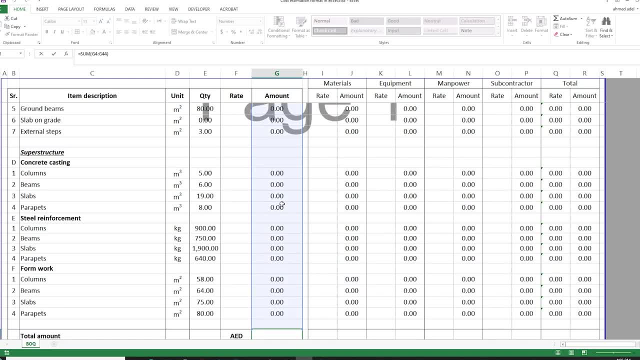 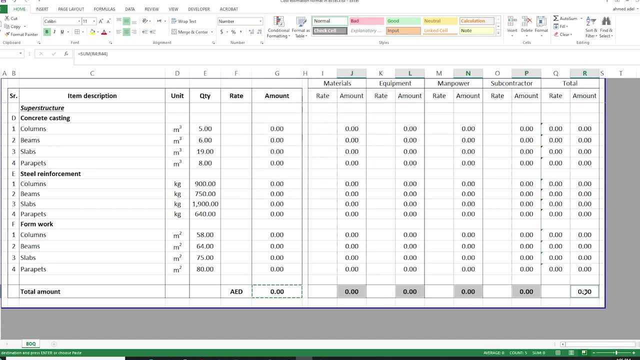 click ok and the same formula that i have here, which is the submission of the column. i also want to know the total amount for each of these cost elements. i want to know how much is the total materials required for the project, how much is the equipment required, how much is the total manpower and how much is the total subcontractor and of. 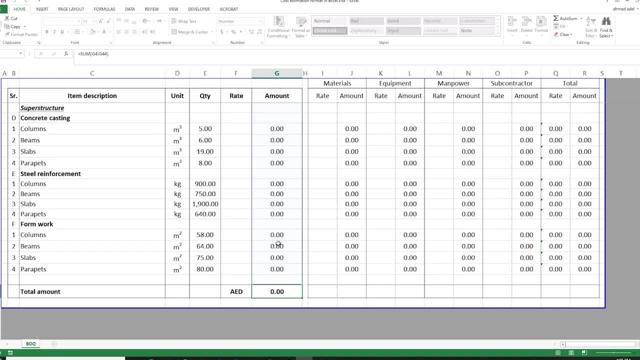 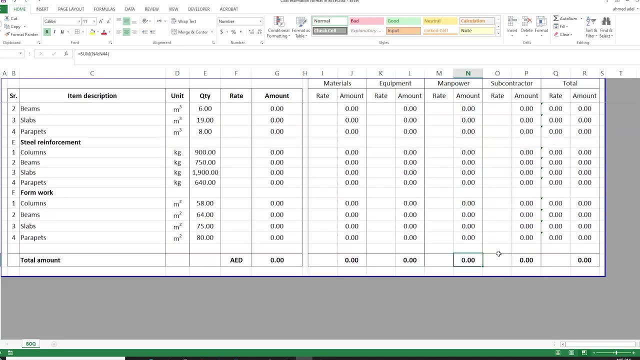 And the same formula that I have here, which is the submission of the column. I also want to know the total amount for each of these cost elements. I want to know how much is the total materials required for the project, how much is the total equipment required, how much is the total manpower and how much is the 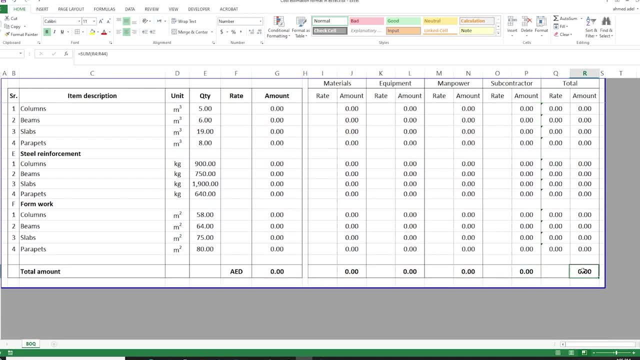 total subcontractor And, of course, here the total amount here if you will use, if you will put this cost rate, the same cost rate, total cost rate here, if you will put it here, then the amount you get in the BOQ is similar to the amount, the total amount, that you get here. 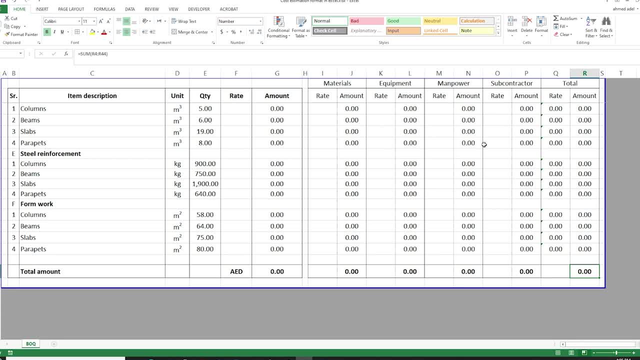 course, here the total amount here, if you will use, if you will put this cost rate, the same cost rate, total cost rate here, if you will put it here, then the amount you get in the voq is similar to the amount, the total amount, that you get here. but usually what happens? we estimate the cost on 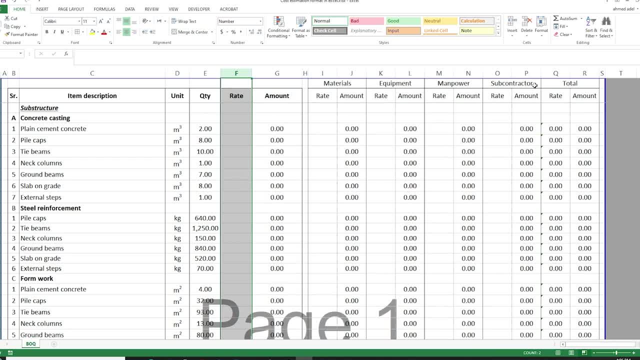 this side, and then we put our ceiling rate here, which means this rate plus the margins that we need. this is something that we can talk about later, but this is how we can do or calculate this format now. the next part is: if you are estimating the cost, you will have another tabs here. you will 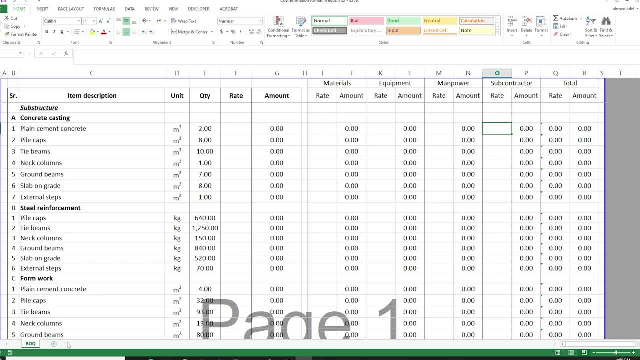 have the material tab and you will have your labor productivity and activity cost tab and all of these things. so you will start linking these cells to your other tabs where you have estimated the costs of the manpower and if you have some material sheet and some subcontractor. 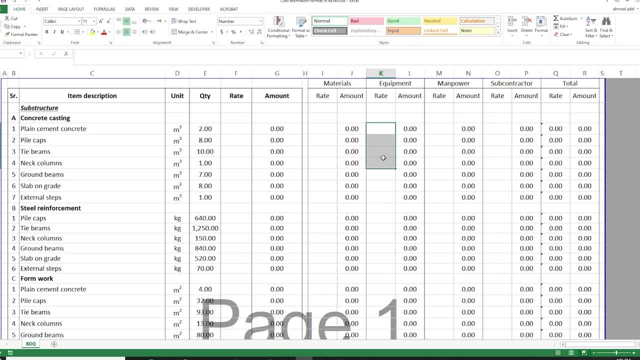 equipment sheet and so on. i have done this in details in our cost estimation course, but now just to run the formulas, let me put some numbers here to make it quick and to show you how the formulas work in that case. so when we are talking about concrete casting, i have only the materials. 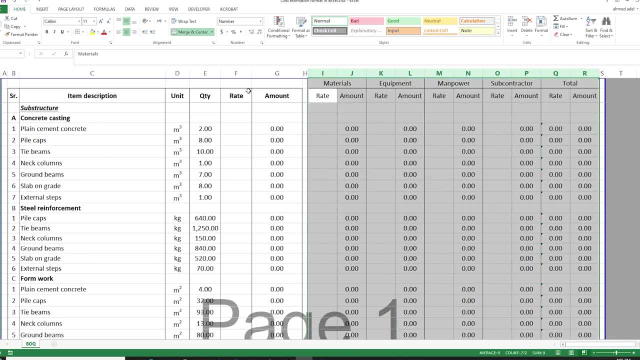 But usually what happens? we estimate the cost on this side and then we put our ceiling rate here, which means this rate plus the margins that we need. This is something that we can talk about later, But this is how we can. We can do or calculate this format. 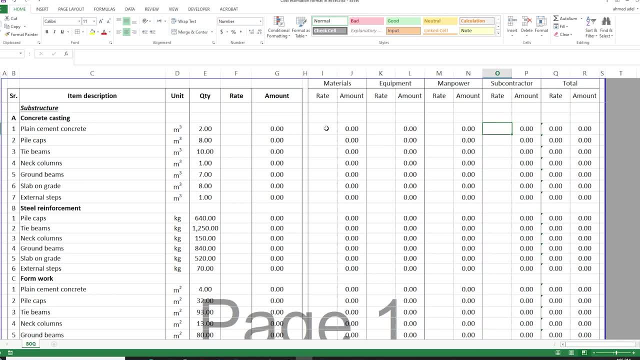 Now the next part is: if you are estimating the cost, you will have another tabs here. You will have the material tab and you will have your labor productivity and activity cost tab and all of these things. So you will start linking these cells to your other tabs where you have estimated the costs of the manpower. 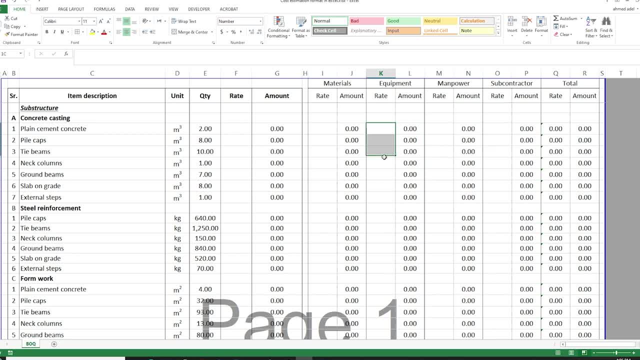 And if you have some material sheet and some subcontractor sheet, some equipment sheet and so on. I have done this in details, in our cost estimation, Of course, but now just to run the formulas, let me put some numbers here to make it quick and to show you how the formulas work in that case. 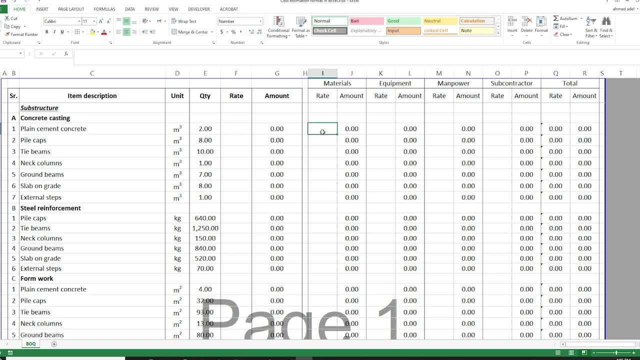 So when we are talking about concrete casting, I have only the materials of the concrete, plus pump, plus ice or plus temperature control. So I'll just put here 250 and the equipment- maybe I have vibrator or something- So I'll just add five dirhams per cubic meter and for the manpower. actually, I have shown in one of the previous videos. 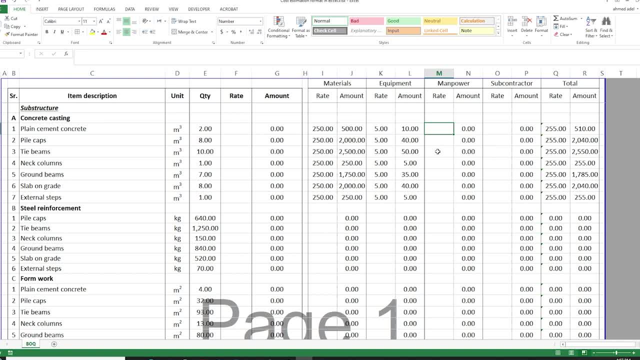 How to calculate the cost for the manpower for each activity in the project. Now, this activity is the concrete casting, So if you haven't watched that video, I'll leave the link in the description. You can go and watch. But this is the manpower cost for the concrete casting. 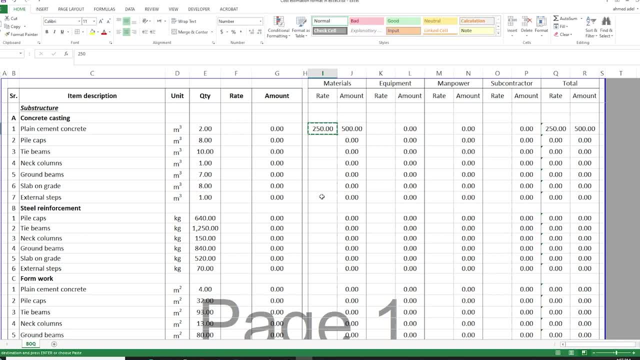 of the concrete, plus pump, plus ice or plus temperature control. so i'll just put here 250. and the equipment- maybe i have vibrator or something. so i'll just add five dirhams per cubic meter. and for the manpower: actually i have shown in one of the previous videos how to calculate the cost for 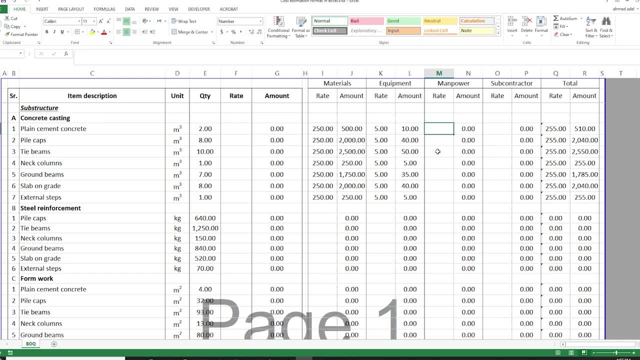 the manpower for each activity in the project. now this activity is the concrete casting. so if you haven't watched that video, i'll leave the link in the description. you can go and watch. but this is the manpower cost for the concrete casting. i'll put here 15. as i told you, you can link these cells. 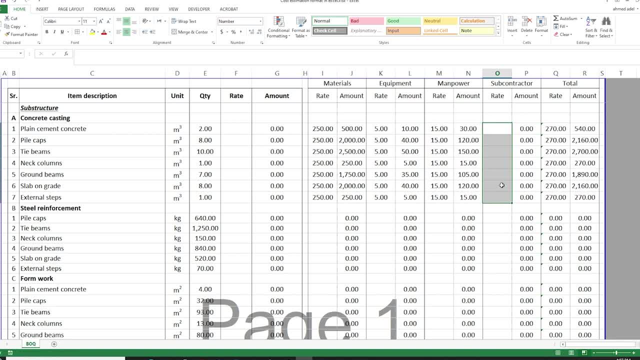 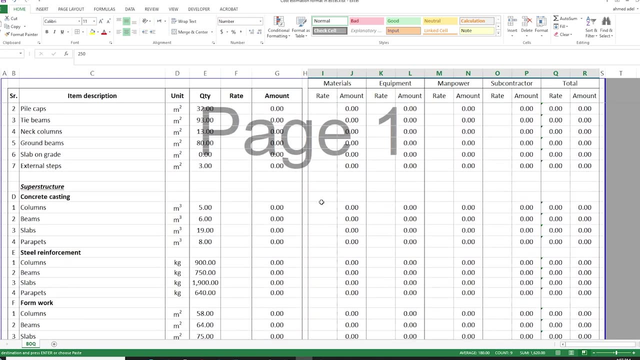 to your other sheets. that's fine, and for the subcontractor: here i don't have anything. so this is how i estimated the cost of the concrete works and actually when i am talking about concrete element, the same exact line. i can take it, because this is for the substructure. i can take the same. 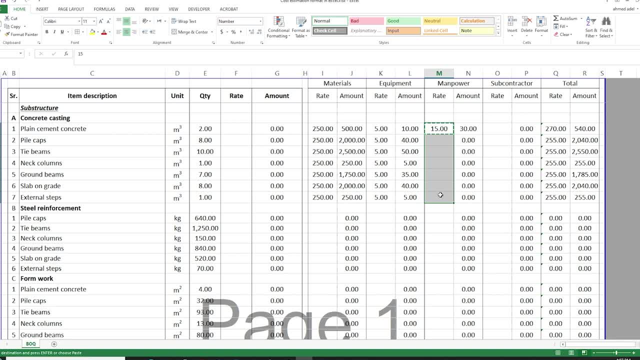 I'll put here 15.. As I told you, you can link these cells to your other sheets. That's fine, And for the subcontractor here I don't have anything. So this is how I estimated the cost of the concrete works. 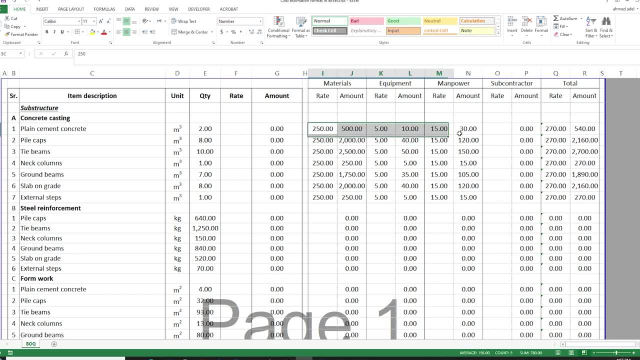 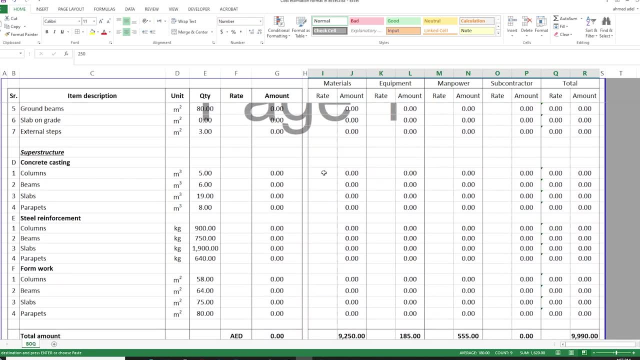 And actually, when I am talking about concrete elements, The same exact line. I can take it because this is for the substructure, I can take the same and go here to the superstructure, and I can face the same because everything is similar. 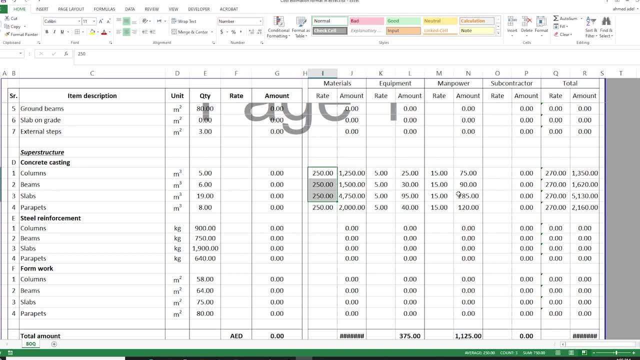 The concrete casting is similar, The equipment similar, The material is same material. Or maybe here let's make it a little bit more expensive. Let's put it to 60 if the concrete required for the superstructure is more expensive. But usually it is actually less expensive. 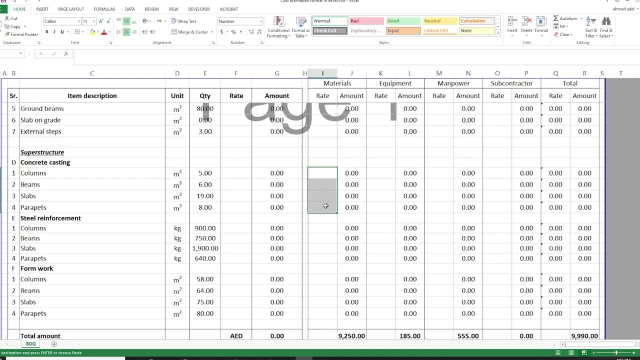 and go here to the superstructure and i can paste the same, because everything is similar: the concrete casting is similar, the equipment similar, the material is same material. or maybe here let's make it a little bit more expensive, let's put it to 60 if the concrete required for the superstructure 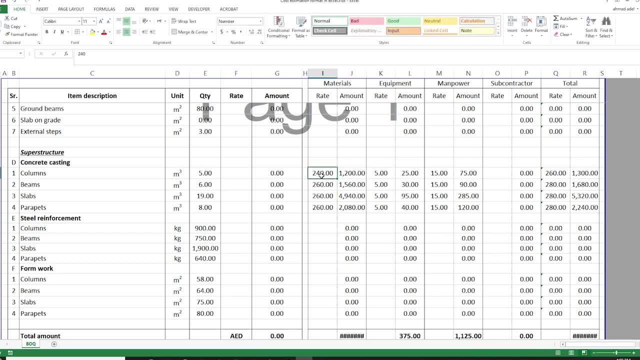 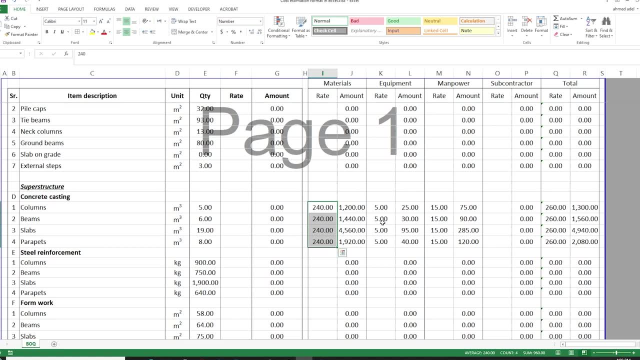 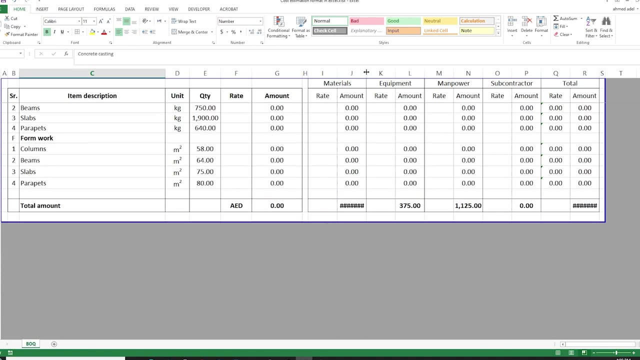 is more expensive, but usually it is actually less expensive. anyway, you will just have here the material rate, equipment rate, manpower rate and subcontractor rate. so now i have finished the estimation for my concrete casting for the superstructure and for the substructure as well, and actually i'm 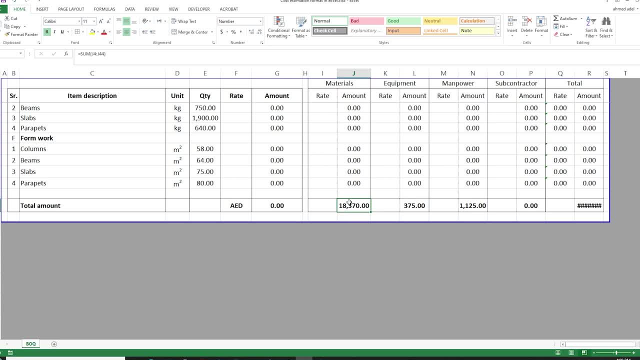 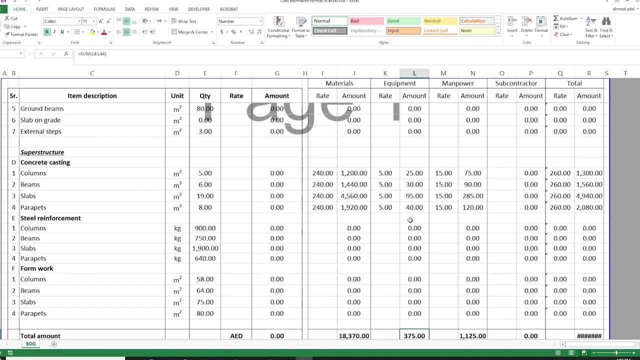 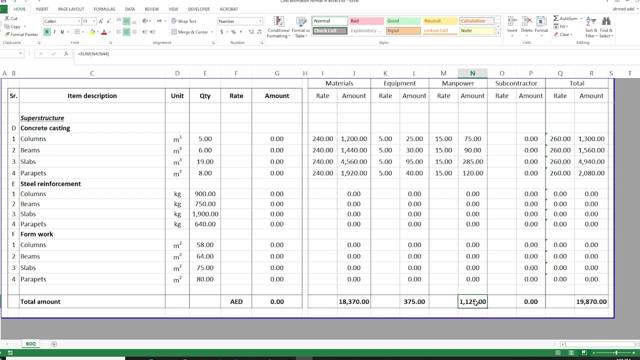 starting to get some amounts here. so i am getting that. i need 18 000 for the supply of concrete here, as you can see, and i am getting here 375 for the equipment, vibrator or whatever. actually, this is a small project or the quantities are very small, so that's why the numbers are small. i need 1100. 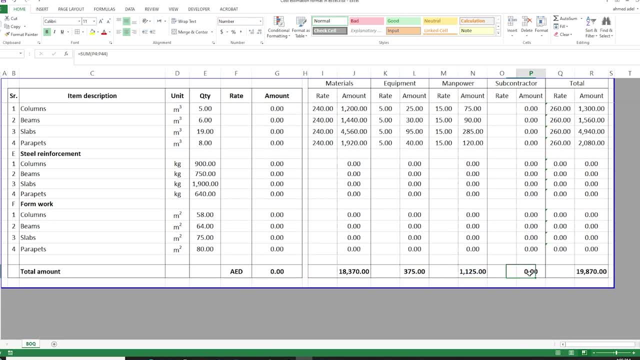 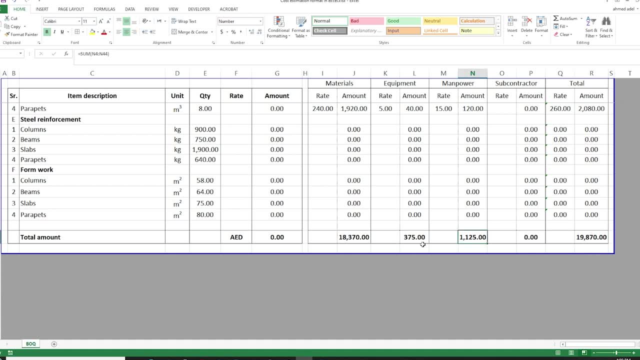 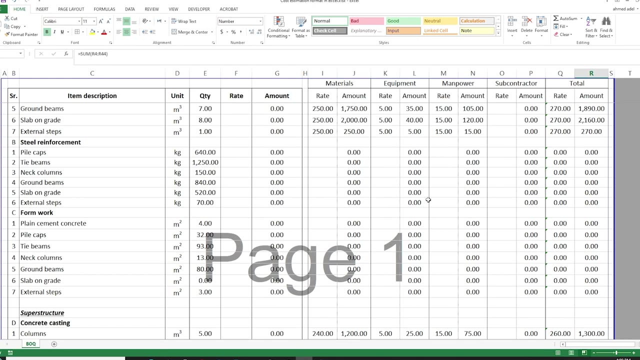 is the cost of manpower that i need to cast the concrete and zero subcontractor, because i i didn't price any subcontractors here and this is the total cost so far, which is this plus this, plus this, plus the subcontractor, which is zero. so the submission of these three is the 19 000 here. so 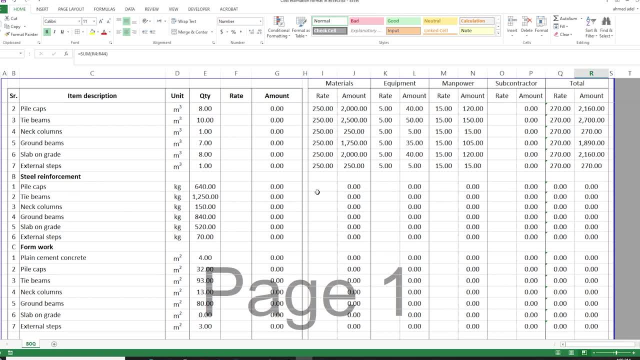 let's continue our estimation now. let's go to the steel reinforcement, for example. so for the materials here the quantity is in kg, so this is the material cost let's have here. per kg let's put something like 3.5 or something. this you will get it from the material rate, depending on the price. 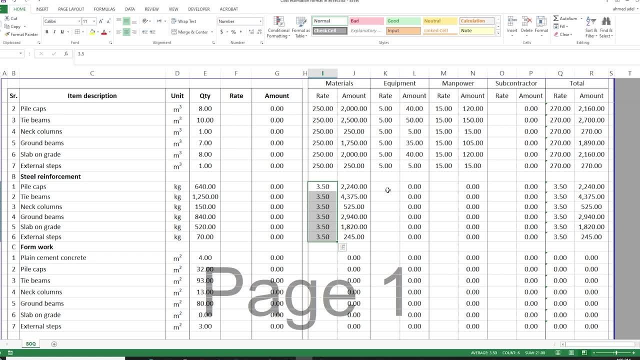 per ton. you will divide that by 1000 to get this rate. then for the equipment i might need some hand tools and so on. so i just can add: let's say let's have it like 0.5 or something. i don't want to make it very expensive. 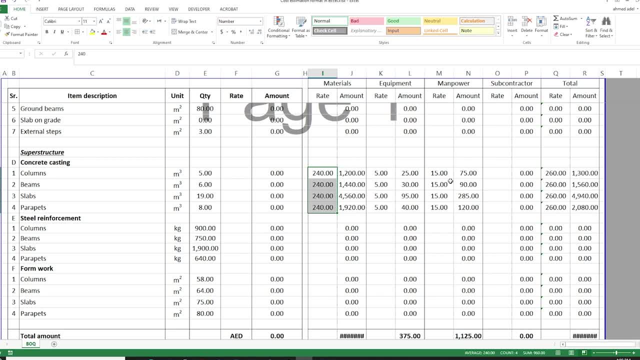 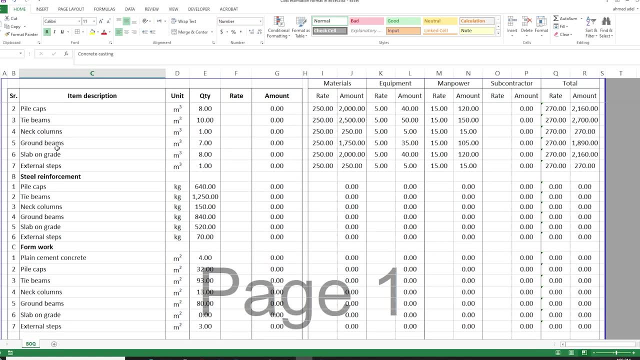 Anyway, you will just have here the material rate, Equipment rate, Manpower rate And subcontractor rate. So now I have finished the estimation for my concrete casting for the superstructure and for the substructure as well, And actually I'm starting to get some amounts here. 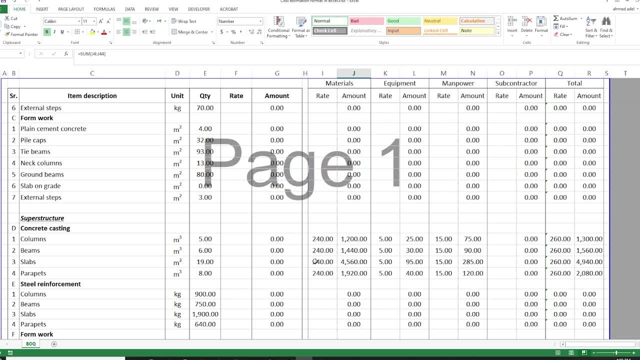 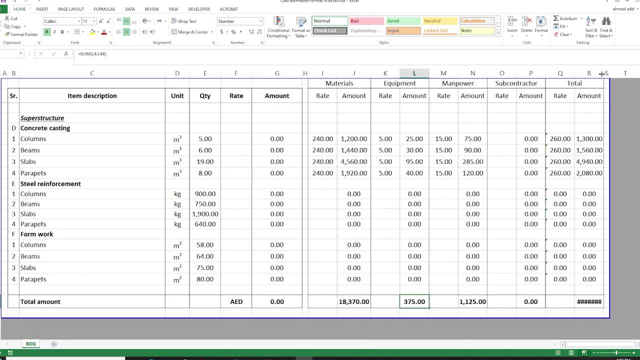 So I am getting that I need 18,000 for the supply of concrete here, as you can see, And I am getting here 375 for the equipment, vibrator or whatever. Actually, this is a small project or the quantities are very small. 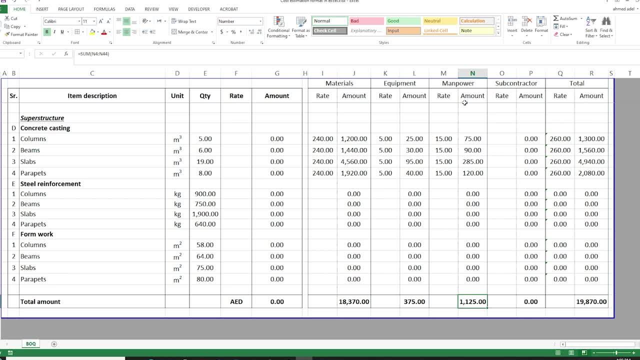 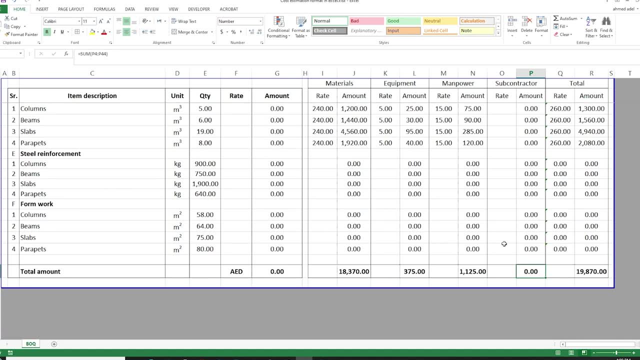 That's why the numbers are small. I need 1100.. This is the cost of manpower that I need to cast the concrete and zero subcontractor, because I didn't price any subcontractors here. And this is the total cost so far, which is this plus this, plus this plus the subcontractor, which is zero. 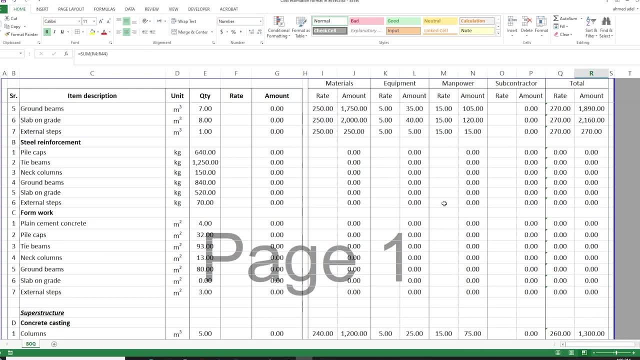 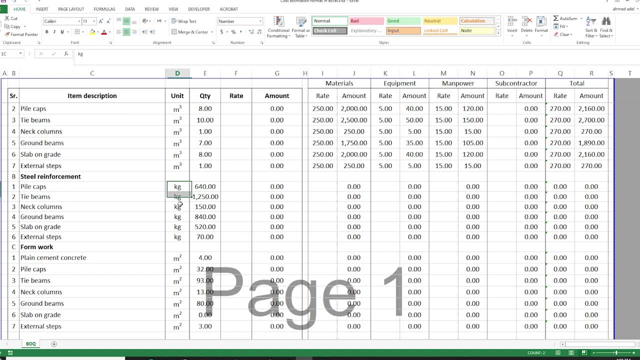 So the submission of these three is the 19,000 here. So let's continue our estimation. now Let's go to the steel reinforcement, for example. So for the materials here the quantity is in kg, So this is the material cost. 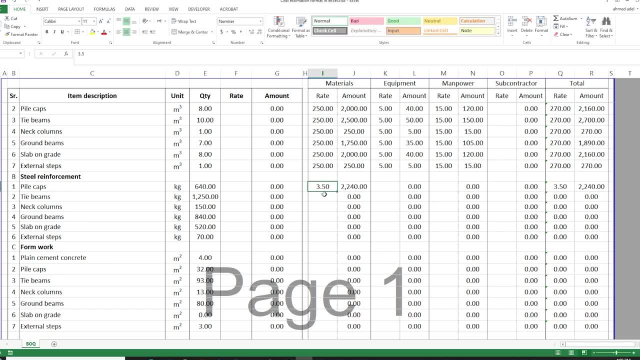 Let's have here per kg. Let's put Something like 3.5 or something. This you will get it from the material rate, depending on the price per ton. You will divide that by 1000 to get this rate. Then for the equipment, I might need some hand tools and so on. 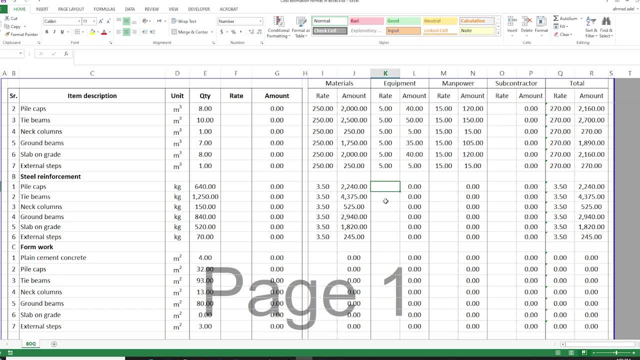 So I just can add: let's say, let's have it like 0.5 or something. I don't want to make it very expensive. OK, because this is in each kilogram. I am assuming 0.5, actually 0.5 seems to be a little bit high. 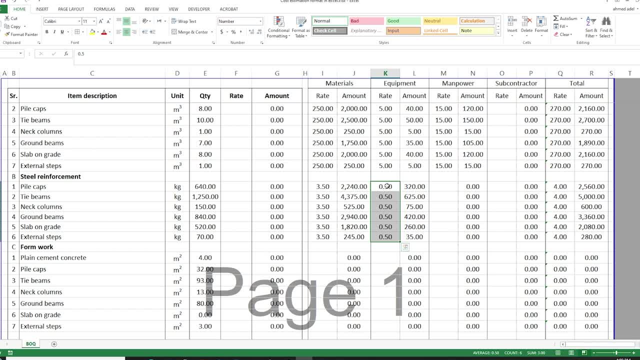 okay, because this is in each kilogram. i am assuming 0.5. actually 0.5 seems to be a little bit high for me, and then after that is still fixing how much was the rate per kilogram? we can have 0.4 and 0.4. 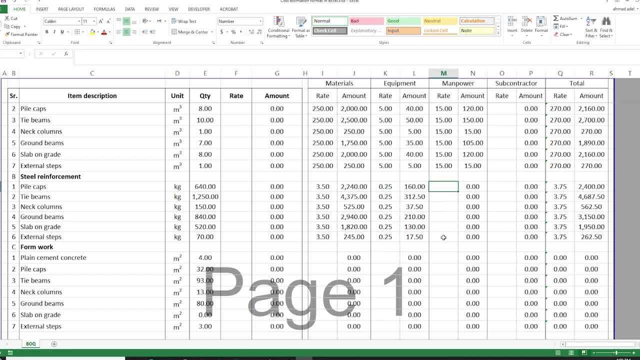 For me, And then after that is still fixing, how much was the rate per kilogram? We can have 0.4 and 0.4 for all of them, So I am getting a total cost for the steel here about 4.15 per kilogram, which is a little. 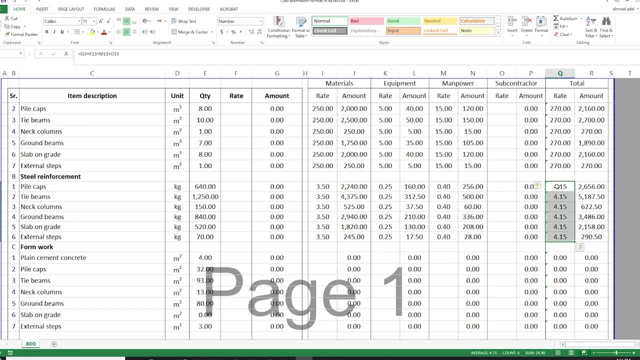 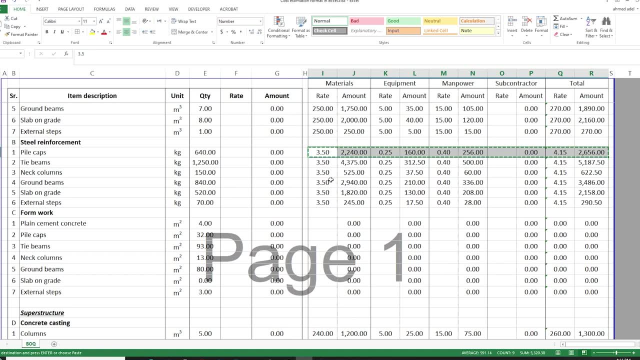 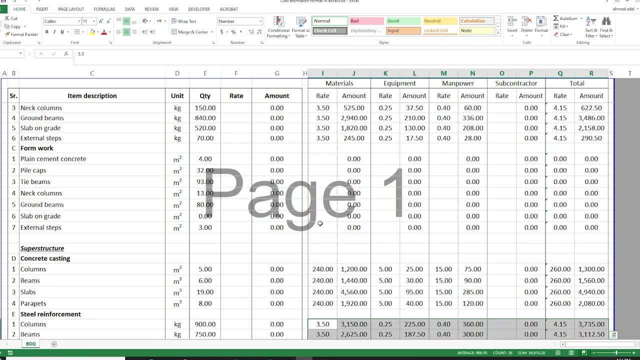 for all of them. so i am getting a total cost for the steel here about 4.15 per kilogram, which is a lot, and, as we said, we can copy this because it's a steel reinforcement, and i'll price the steel reinforcement of the superstructure as well. then after that, let's go to the form work and for the 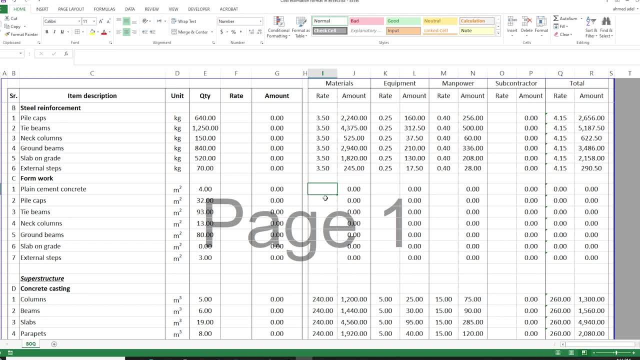 materials for the form work. the materials here will include both the wood that you need- the plywood- and the box sections and everything plus the scaffolding. so of course there is a detailed breakdown for this number, but let me have it here as 18. let's say i'll just have 18 and then i'll have 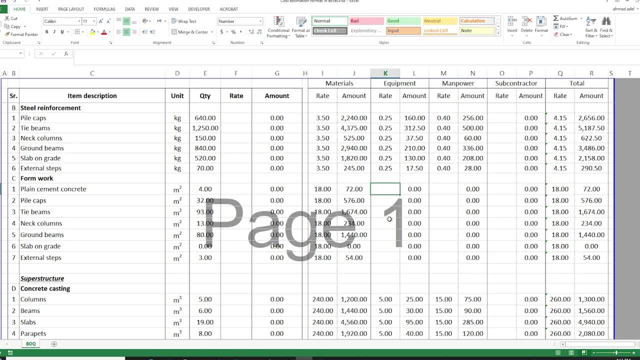 18 here, and then for the equipment for the form work, again some hand tools and so on. so let's just have two dirhams or something for the hand tools and the manpower, which is the manpower for the form work. so one second. let me calculate it. so 12 dirhams here. 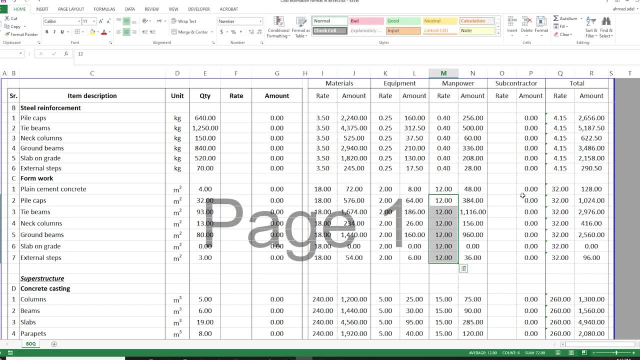 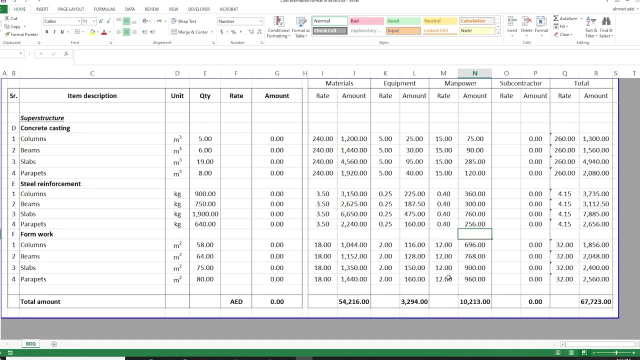 and the rate. the total rate that i am getting as a cost here is 32 for the form work. so i can copy. i can price the form work here as well. okay, so now i started to get some numbers. as you can see here, i am getting 55 000 almost for the. 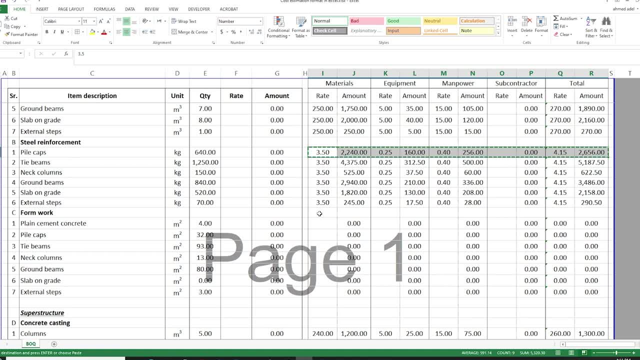 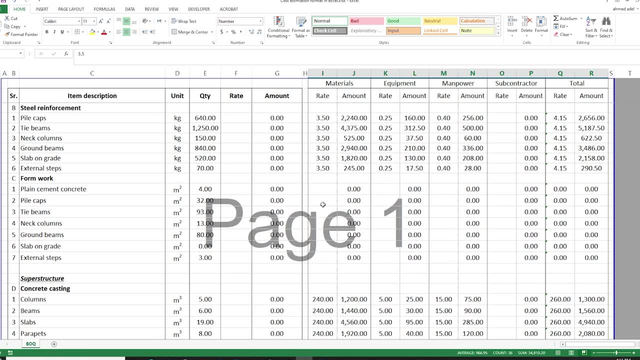 bit logic And, as we said, we can copy this, because it's a steel reinforcement and I'll price the steel reinforcement Of the superstructure as well. Then, after that, let's go to the formwork, and for the materials, for the formwork, the 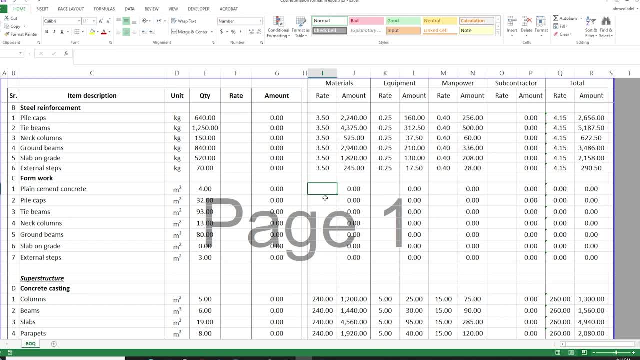 materials here will include both the wood that you need, the plywood, and the box sections and everything plus the scaffolding. So of course there is a detailed breakdown for this number, but let me have it here as 18.. Let's say I'll just have 18 here, and then for the equipment, for the formwork again. 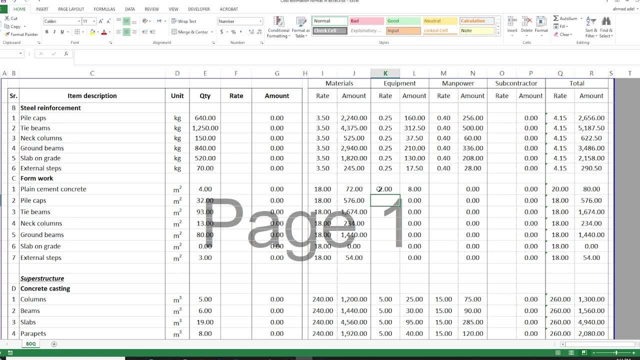 some hand tools and so on. So let's just have two dirhams or something for the hand tools and the manpower which is the manpower for the formwork. So one second. let me calculate it. So 12 dirhams here. 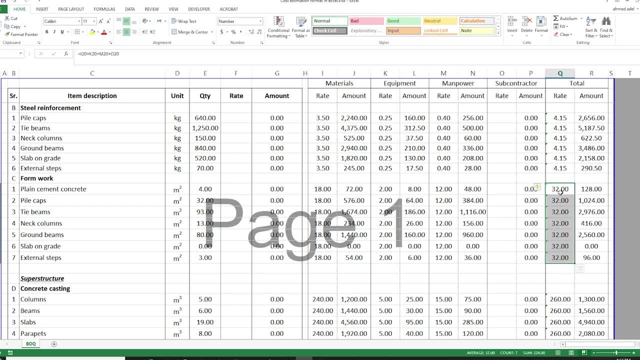 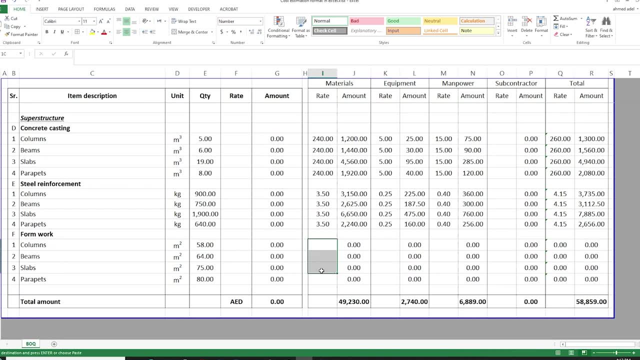 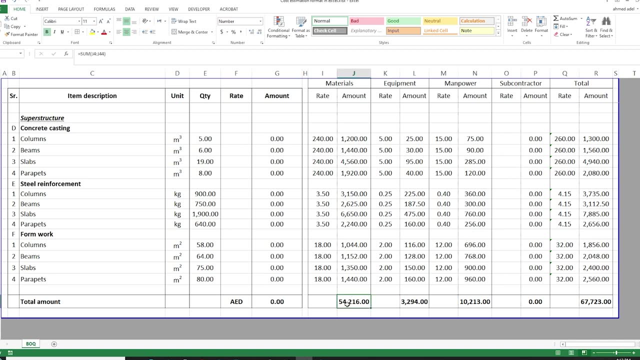 And the rate. the total rate that I am getting as a cost here is 32 for the formwork, So I can copy that and I can price the formwork here as well. Okay, So now I started to get some numbers. As you can see here, I am getting 55,000 almost. for the materials I am getting like 3,300. 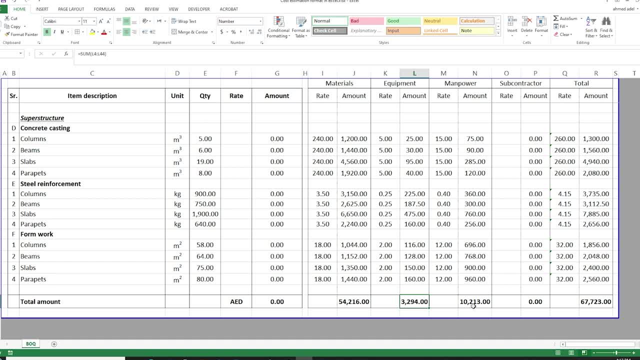 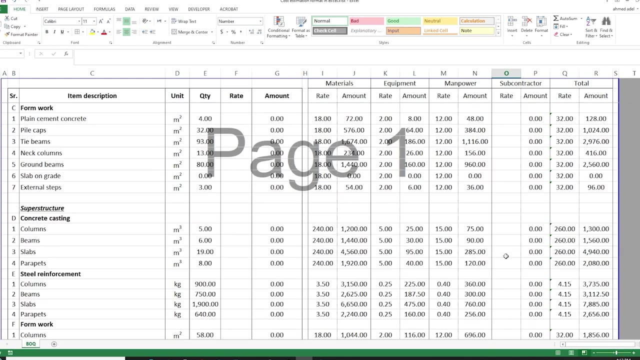 materials. i am getting like 3300 for the equipment and 10 000 for the manpower. that are carpenters, steel fixers and laborers required to do the casting and everything, and i have assumed that i'll do everything in-house, so there is no any subcontractor involved. that's why the 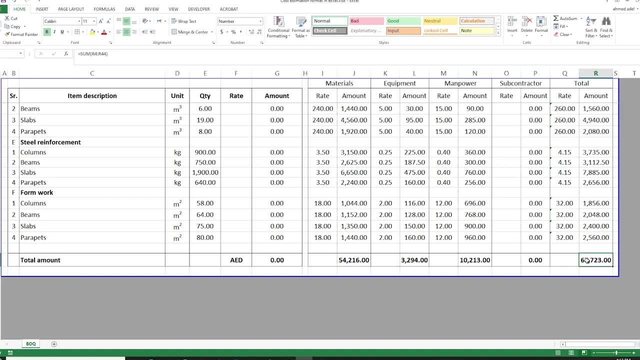 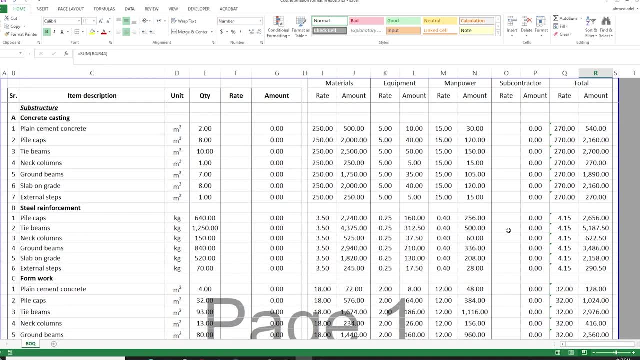 contractor here is zero and i am getting a total cost of 67 000 to execute the concrete works of this project. so this is how you do this sheet. this sheet is actually very useful because, as you can see now, if i want the voq to be equal to the cost, so i'll just make equal to and i can take this rate. 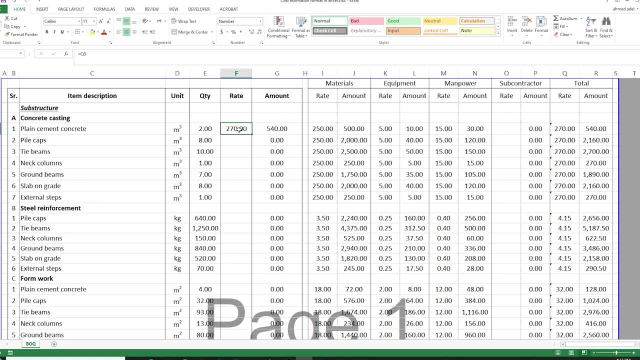 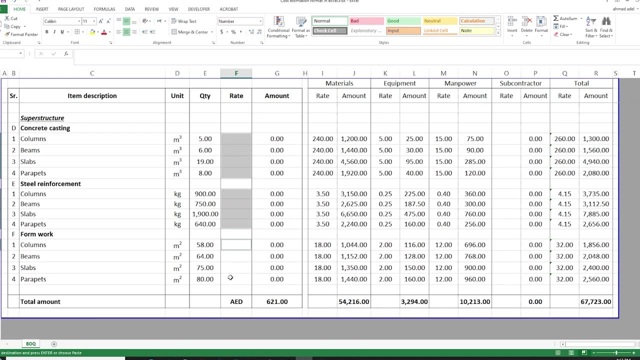 and have it here. but of course, or i can say: let's add, for example, 15, so 1.15, into the total cost rate. i'll just copy this and apply here. okay, so i got my voq now, which is 77 000, and i can mark this all and hide it and i'll print this as a 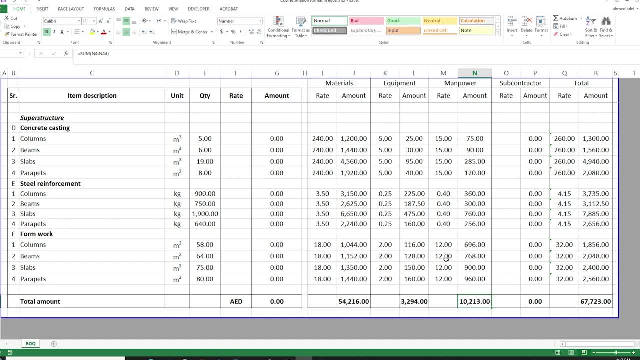 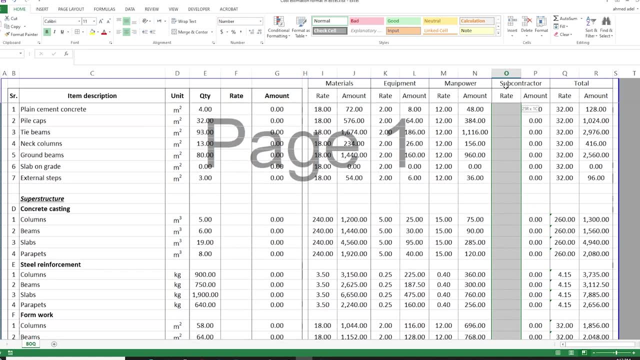 for the equipment and 10,000 for the manpower that are carpenters, steel fixers and laborers required to do the casting and everything. And I have assumed that I'll do everything in house, So there is no any subcontractor involved. 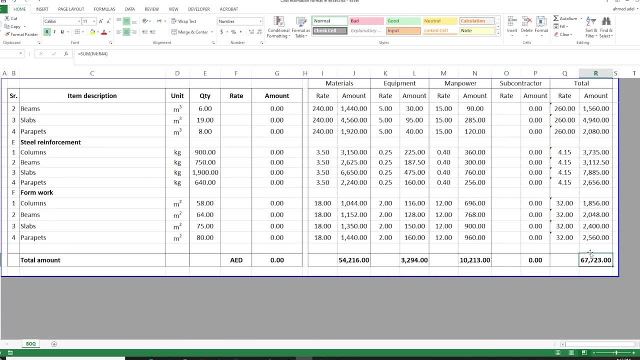 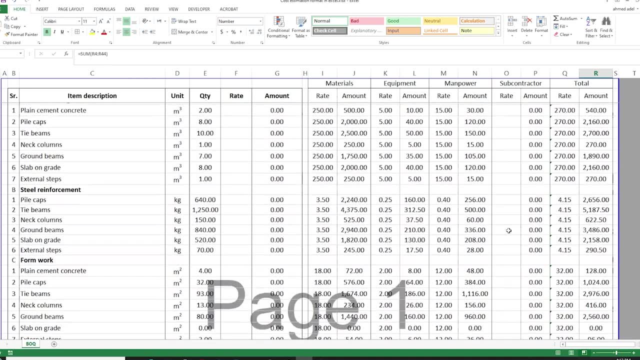 That's why the subcontractor here is zero And I am getting a total cost of 67,000.. Okay, Okay, So I am going to execute the concrete works of this project. So this is how you do this sheet. This sheet is actually very useful because, as you can see now, if I want the BOQ to be, 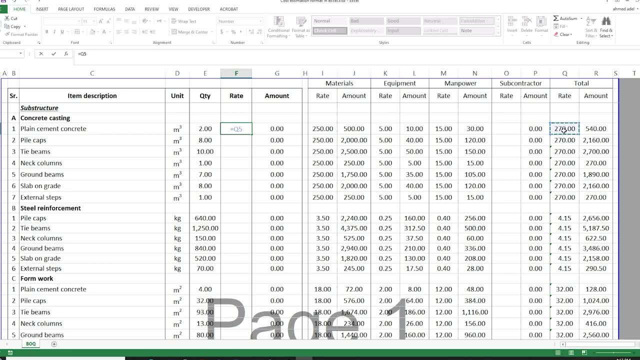 equal to the cost. so I'll just make equal to and I can take this rate and have it here, But of course, or I can say let's add, for example, 15%, So 1.15 into the total cost rate.